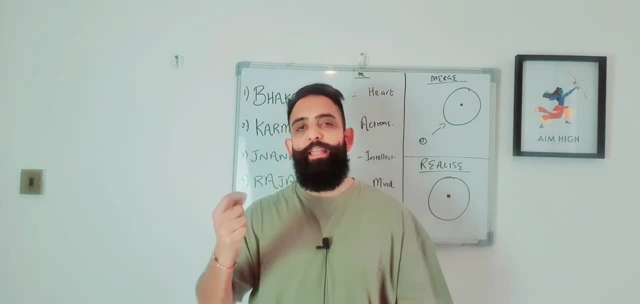 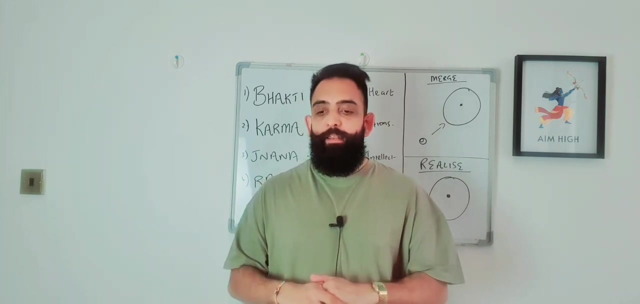 modern world. it is a very tiny, tiny fraction of what yoga actually is. So if we take a step back and look at what is the aim of yoga, why are we doing any of these practices, even the physical ones, then we can define it and say that yoga, essentially, is the path to enlightenment. 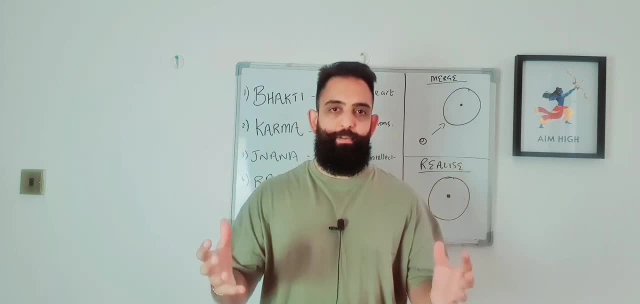 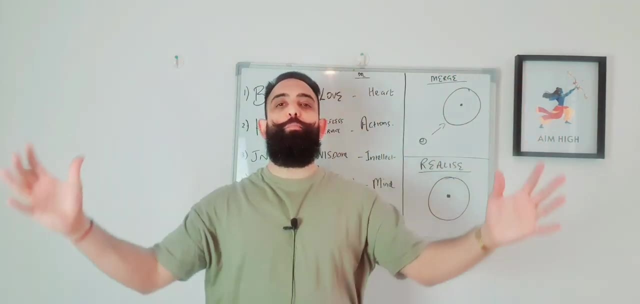 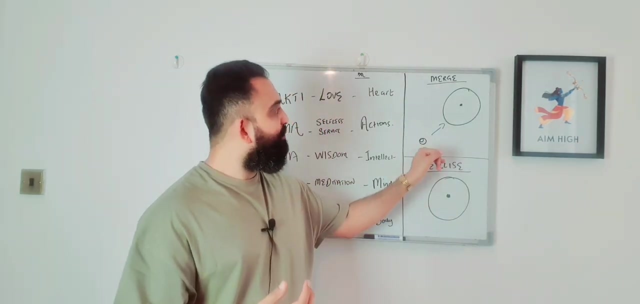 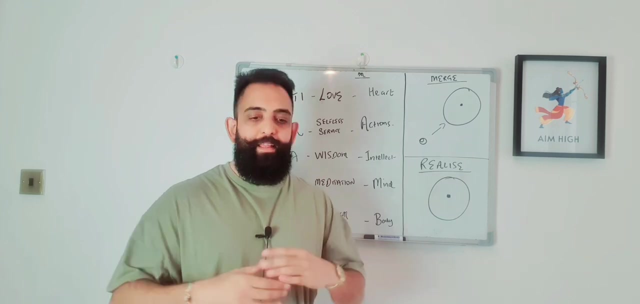 It is the path one can take to enlightenment. It is the path to realizing our true nature as the all-pervading consciousness. It is also the path of uniting our individual consciousness with the universal consciousness. However you want to look at it, the perspective is simply an individual thing, but ultimately, 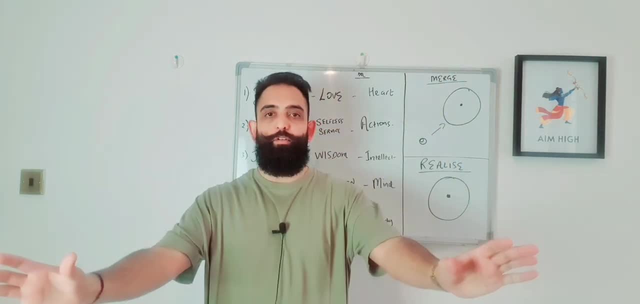 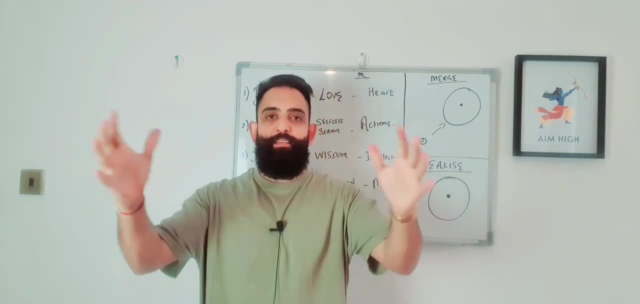 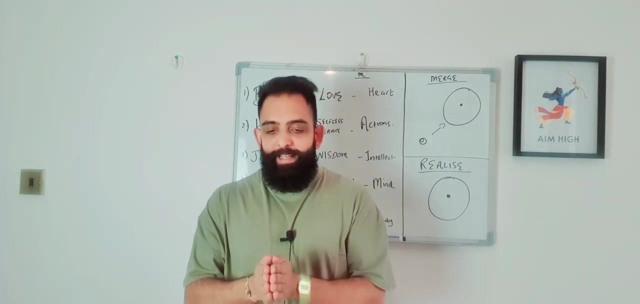 it is to arrive at the main conclusion that we are the universal consciousness, universal consciousness. So if that is the main goal, there is not just one path that will take us there. In fact, there are many different paths that can take us there. Lord Krishna in the Gita. 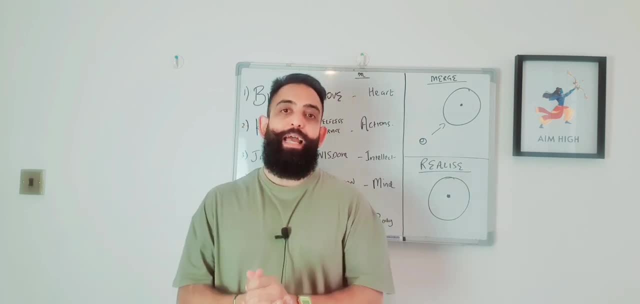 has actually outlined them for us in detail, and today we are going to be discussing the four main types of yoga, and you will be able to see that you can actually pick a path that suits your personality and your temperament. So what that means is that different people have 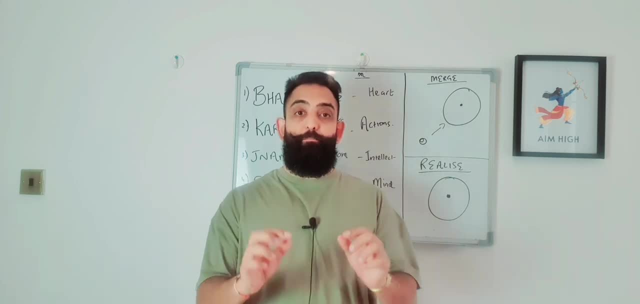 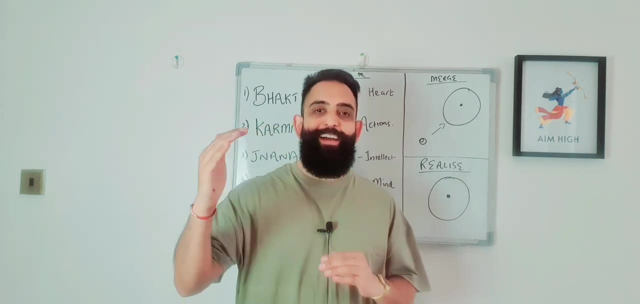 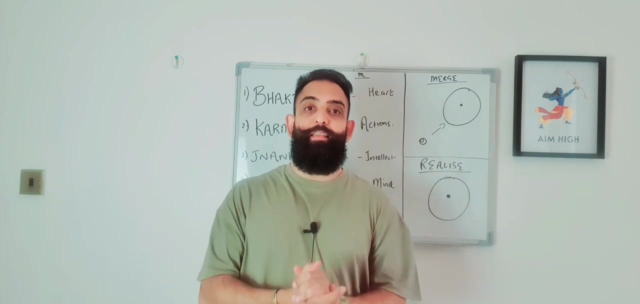 different personalities, different strengths and weaknesses, and based on that, you can choose a path to make the chance of your success much higher. essentially- and that is the beauty of this- There is no one way. There are four main ways, as we'll discuss today, and in these four main ways there are millions of 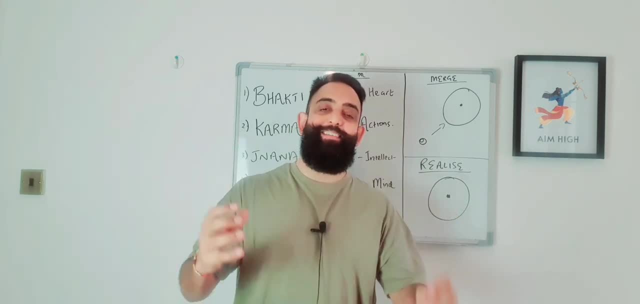 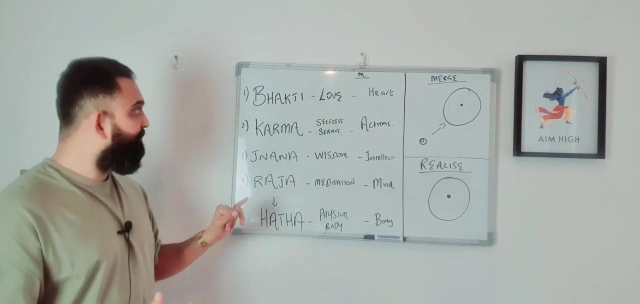 different ways. You can see there are as many ways as there are people in existence, because each one is unique. But let's go and understand the essence of these different paths. So first, listing the different types of yoga, you have Bhakti Yoga, Karma Yoga, Jnana Yoga and Raja Yoga. 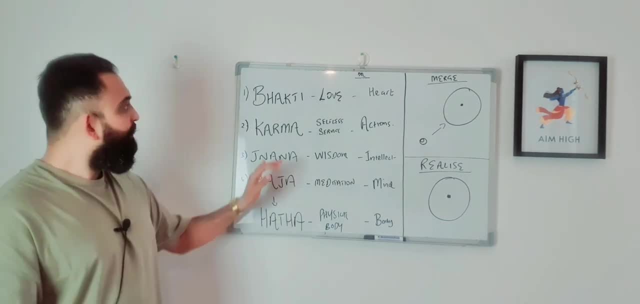 And you can see that there are four main ways, as we'll discuss today, and in these four main ways there are. and then, within Raja Yoga, you have Hatha Yoga. So Bhakti is the path of love, Karma is the path of selfless. 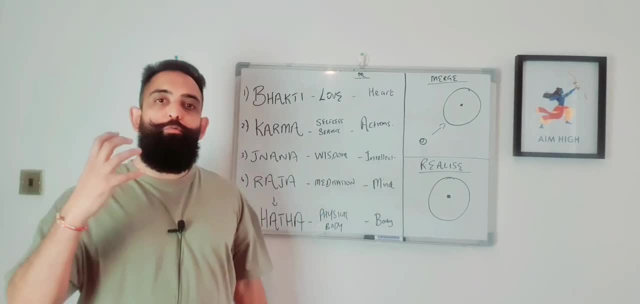 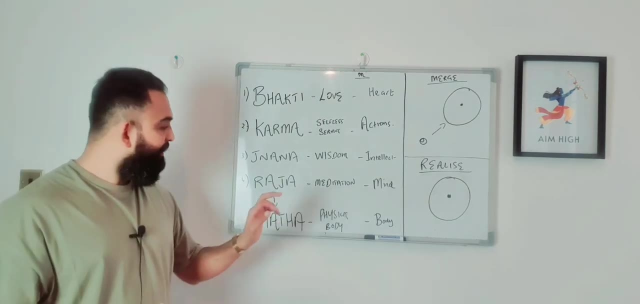 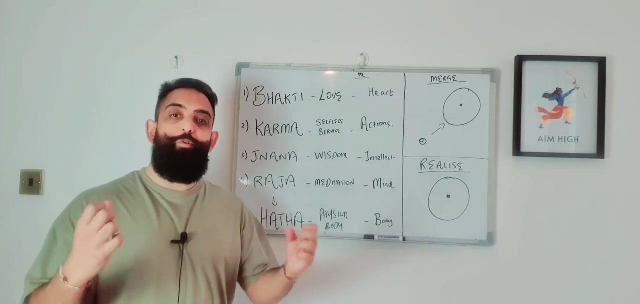 service. Jnana Yoga is the path of wisdom, and Raja Yoga, or the Royal Path, is the path of meditation, And then you have Hatha Yoga, which is the path of the physical body. This is where the physical yoga that we know today actually comes from. 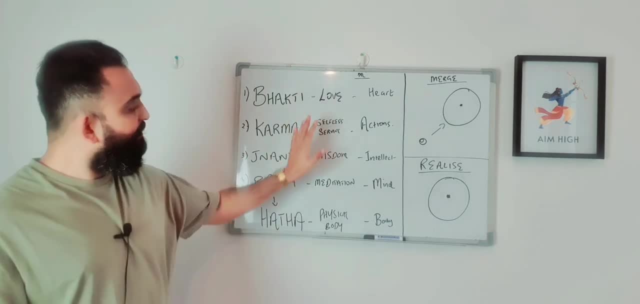 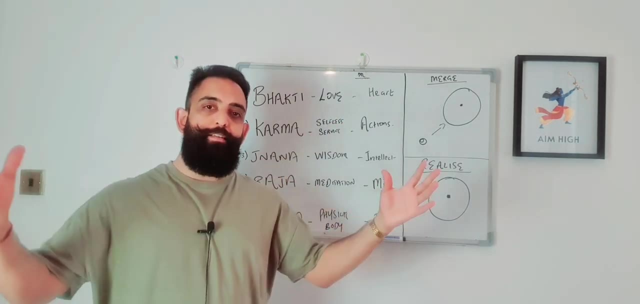 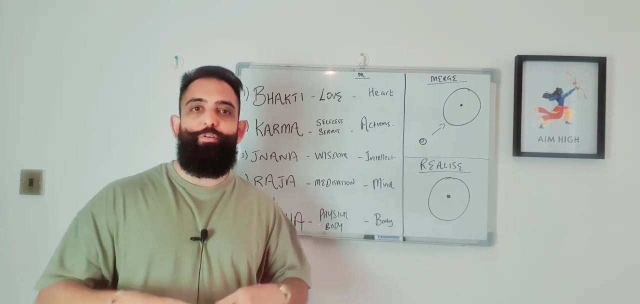 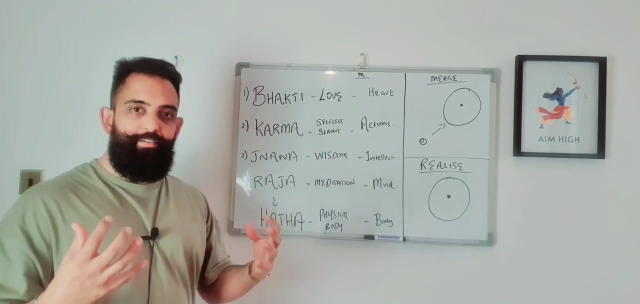 okay, so another way to look at this: right, if we apply another filter on this bhakti, the part of love, we are using our heart to practice this. so if somebody is quite, you know, of an emotional temperament, they are driven by their emotions. this is a great path for them. in karma yoga, it is our actions that are 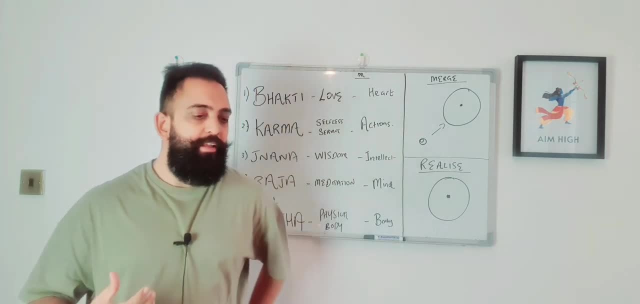 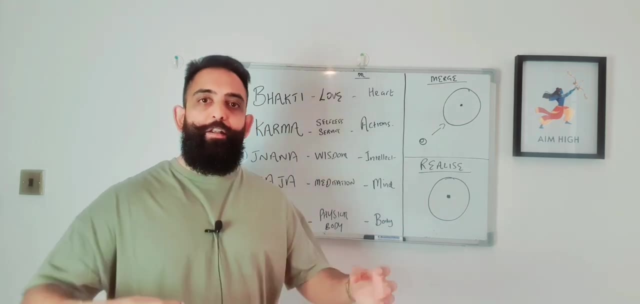 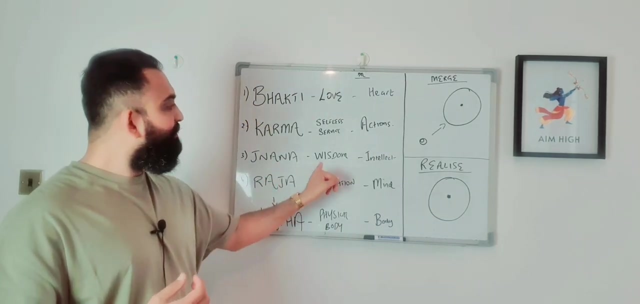 taking charge. so if you are somebody that is very, you know, let's say, hard-working, if you are somebody that is very extroverted, doing a lot of actions, then this can be your path or your main path. Gyan Yoga, wisdom. we are using our intellect, essentially. so if you are somebody who is an intellectual, you love. 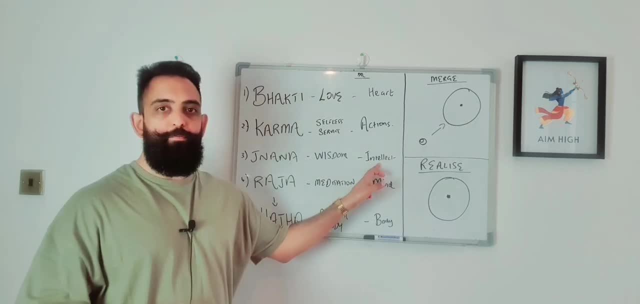 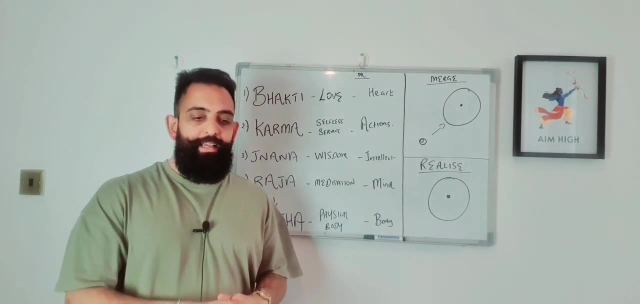 to inquire into things, then this is a path for you. Raja yoga is the path of meditation, and here are the three main paths for meditation and for space based meditation. here we use our mind. So if you are somebody that essentially has a very strong mind, 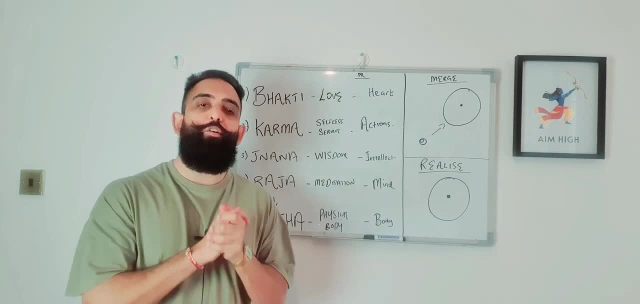 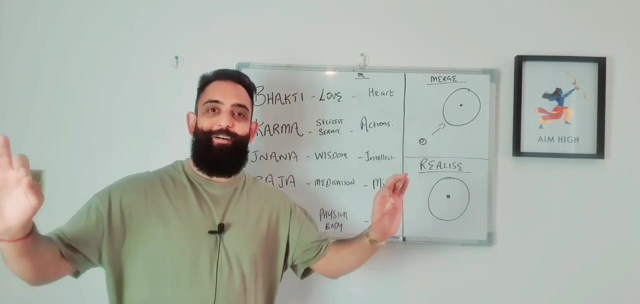 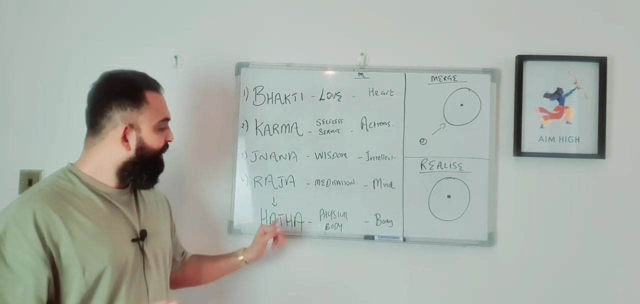 a very strong mind. you know, if you say that from today I'm not going to drink alcohol anymore and that becomes truth, You do not drink alcohol, you know, for the rest of your life. it means your mind is very strong. This can be the main path for you And Hatha Yoga, the part 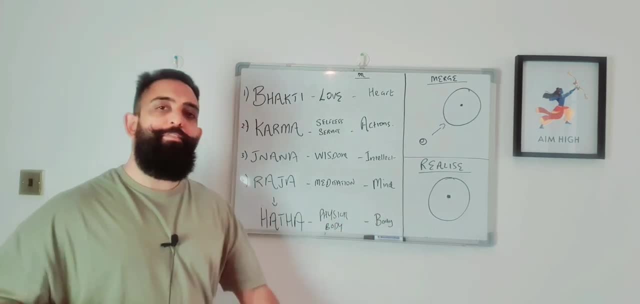 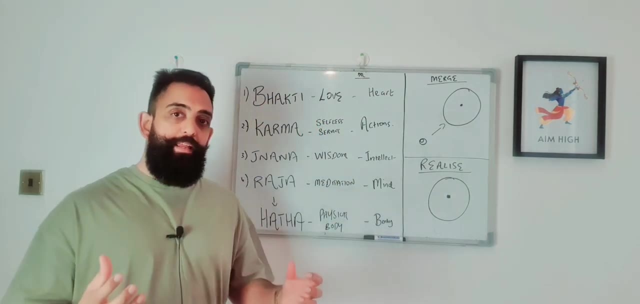 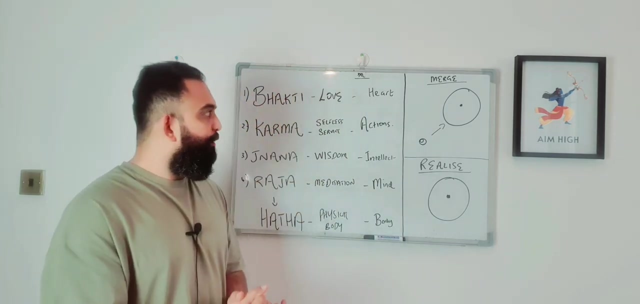 of the physical body. here we are using the body, So if you are somebody that is essentially very athletic, then this can be a main path that you take. So this is again, this is not set in stone, So it doesn't mean that you know, if you are very emotional, you have to take the path of 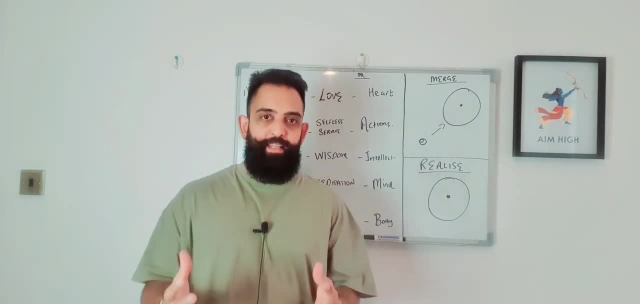 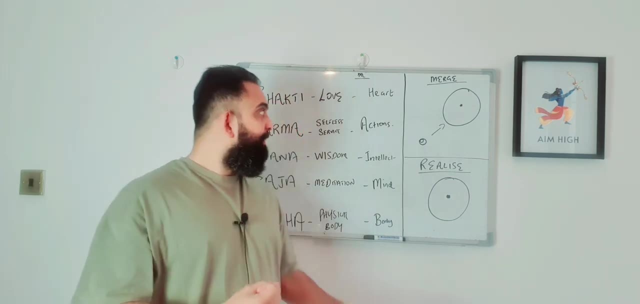 bhakti. That's not what it's saying, But it's giving you a general idea. Okay, so let's go into the definitions of these And it will make a lot more sense. Okay so, in bhakti yoga, bhakti yoga, the path of love, essentially. So here, what is happening is: 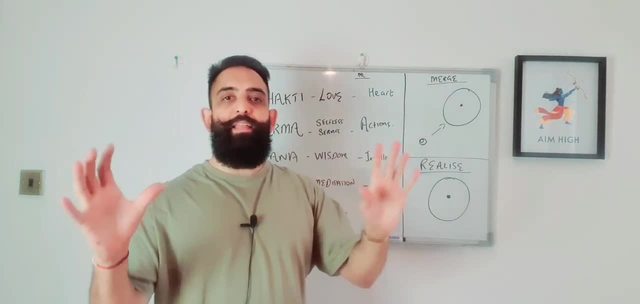 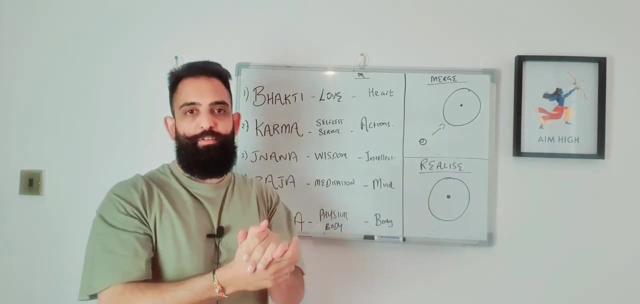 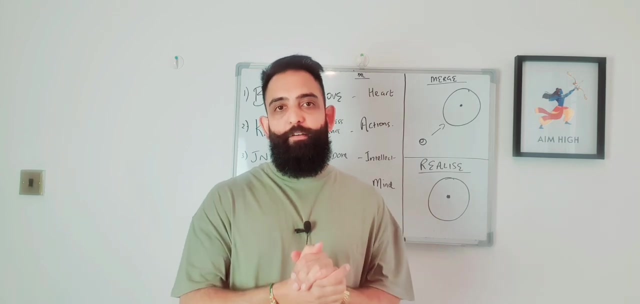 it is actually a path of trying to merge. So you were saying that I am. I am a separate individual entity And there is the universal consciousness And the universal, the universal consciousness is in the form of a personal God that you have, So this could be your Rama, your Krishna. 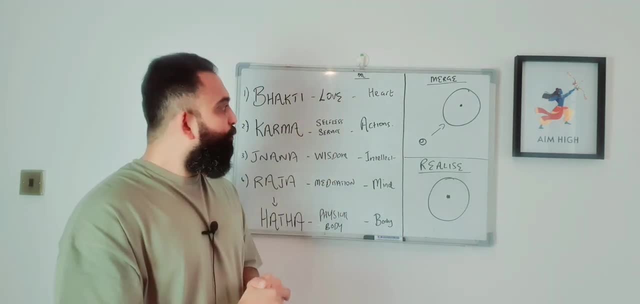 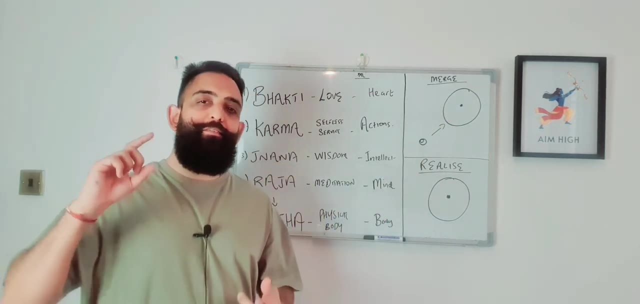 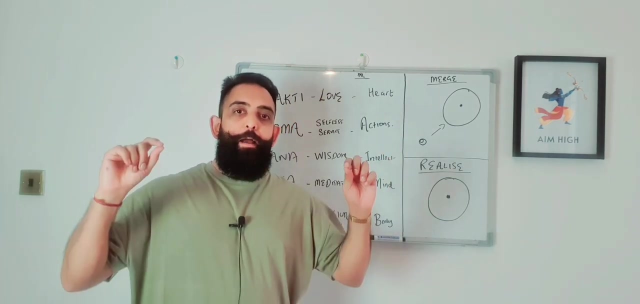 your Allah or Jesus, And what you are saying here is that you are directing all your love toward this deity through means of worship, prayer, singing, bhajan kirtan japa, meditation. whatever it may be, But at the same. 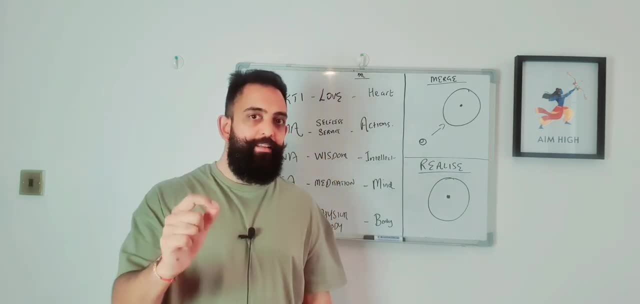 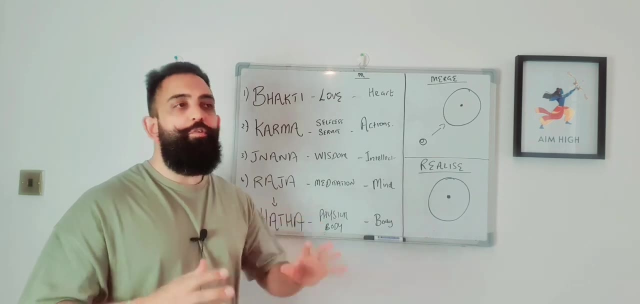 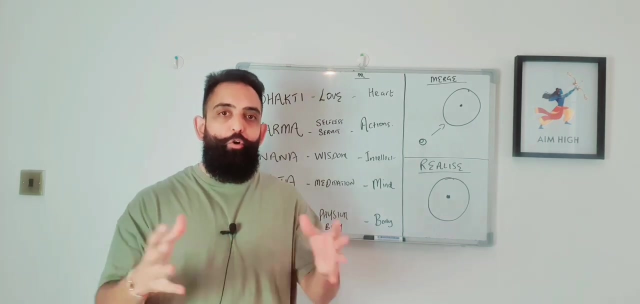 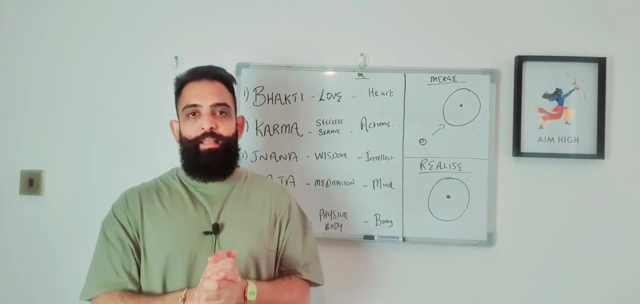 time you are realizing that this deity that I'm praying to, this universal consciousness that I'm praying to, is actually not just a separate entity. it is within all beings, And I need to realize and see all beings as a manifestation of my deity, of my personal God, And 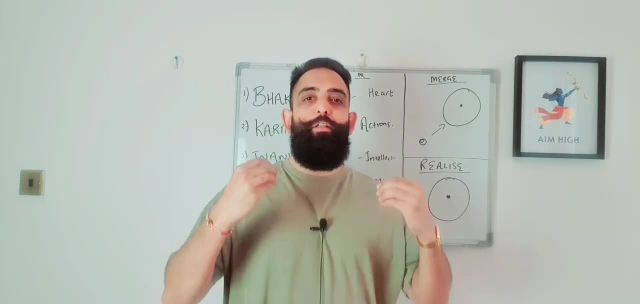 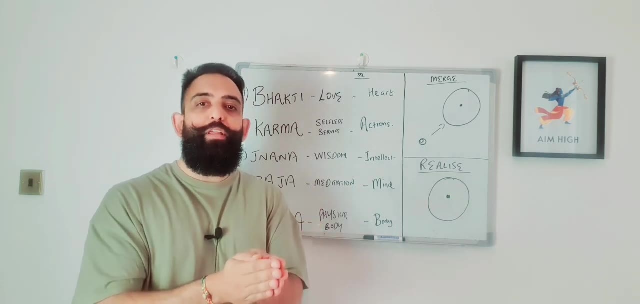 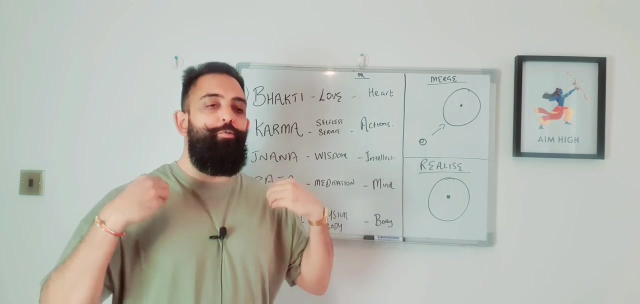 that is true, bhakti. essentially, you are directing your love to this personal aspect of God, And by realizing that he or she is within all children- sorry, all people, or all are his children- you are essentially directing your love toward them as well. 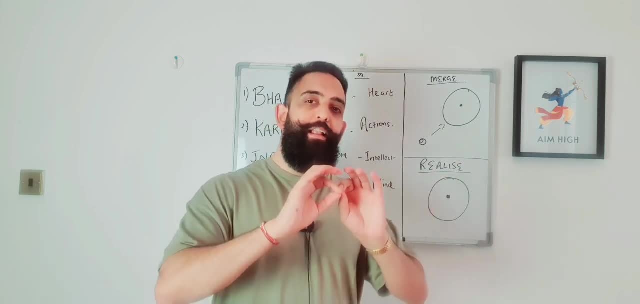 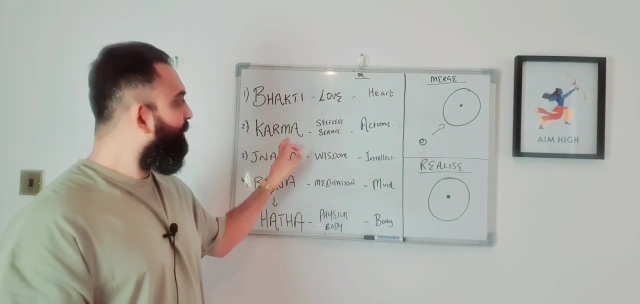 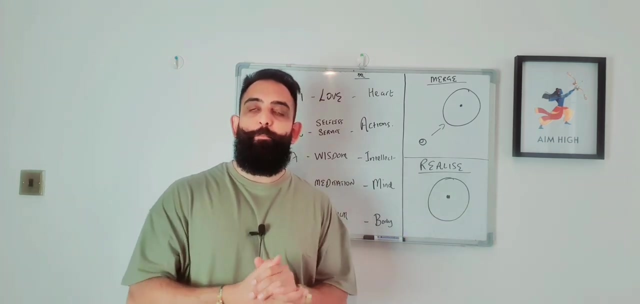 So on this part, this is the part of love, complete love and complete surrender. I hope that makes sense. Then you have the part of Karma yoga, selfless service. So remember what we are trying to do. you know, in the yoga philosophy we covered that. 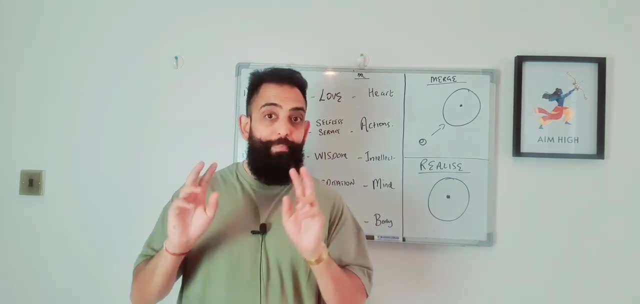 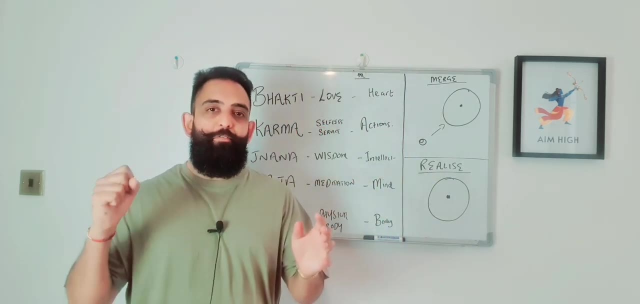 it is because of our ego. this ego is not a bad thing, But the ego is the sense of individuality that keeps us from knowing that, that we are not individuals. we are the all-pervading consciousness, right. So the ego is very high. 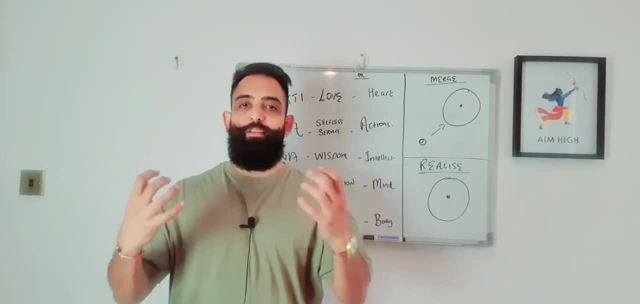 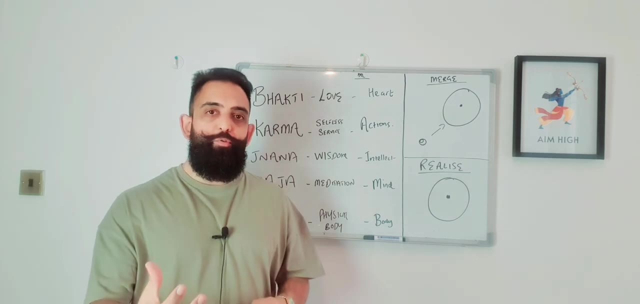 So in Karma Yoga, the premise is that because of my ego, because of my self-sense of individuality, I have become somebody who is very selfish. Anything I do, I'm trying to do it for myself. I'm trying to work for myself, trying to feed myself. 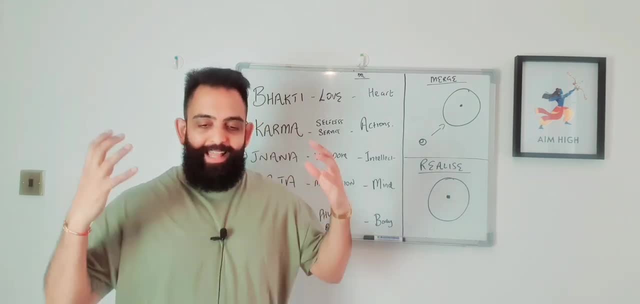 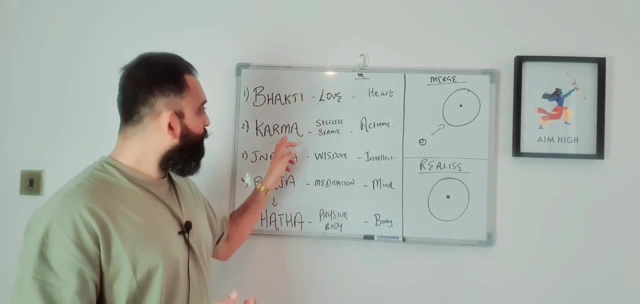 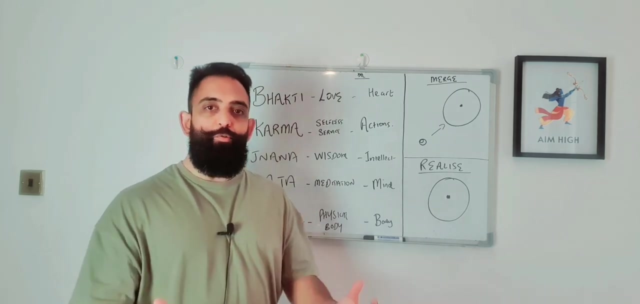 I'm trying to become rich myself. Everything is to please an aspect of our body or somebody in our family. This is how we are as human beings. So in Karma Yoga we are taking the opposite approach. We are saying that through my actions, any action that I do, 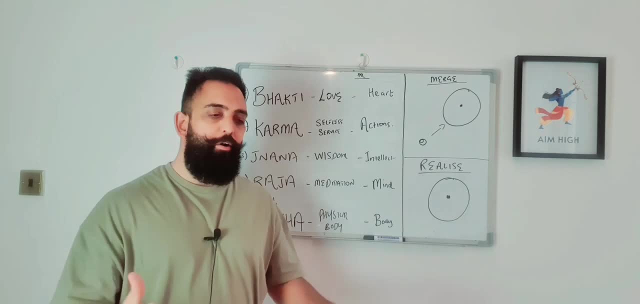 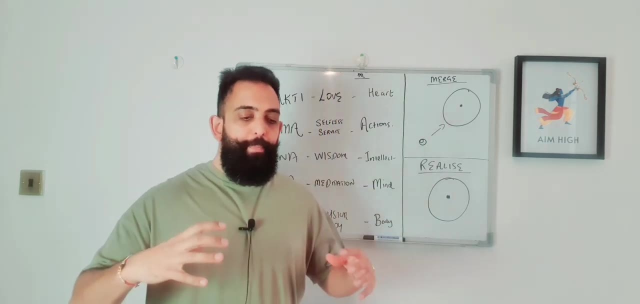 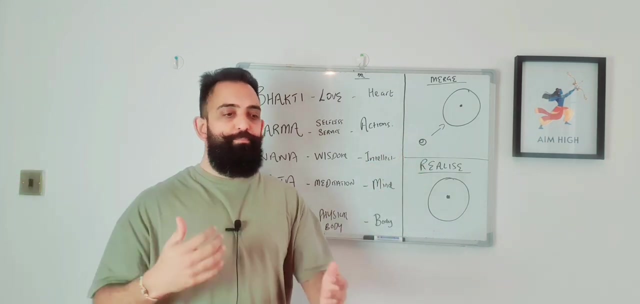 I am giving up the want of the result or the fruit of that action And instead what I'm going to do is I'm going to make my actions an offering to the divine, essentially, So you remove any kind of want from the actions you're doing. 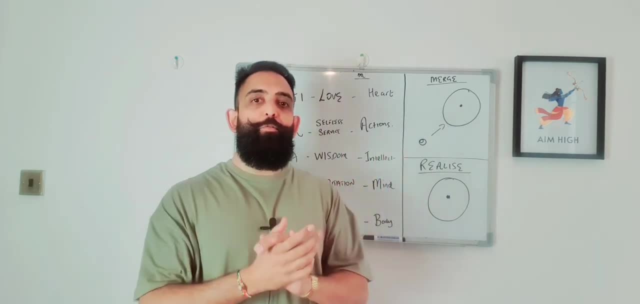 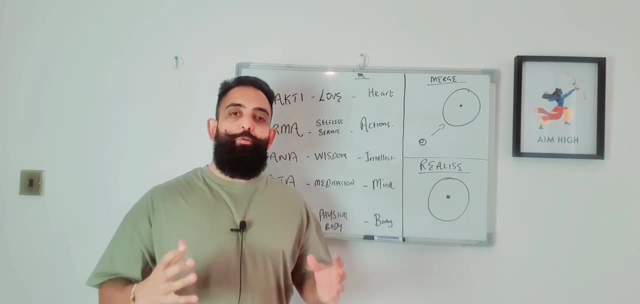 You do all your actions. You do all your actions as an offering. So in Bhakti Yoga, if you remember, we said that your personal aspect of God. you are seeing him or her in all of humanity, in all creatures, in the entire nature. 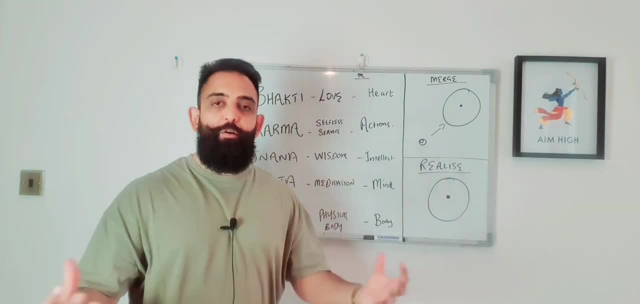 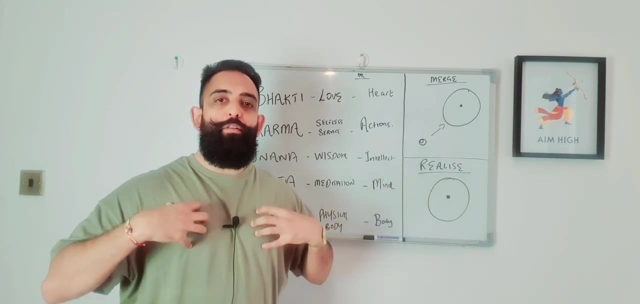 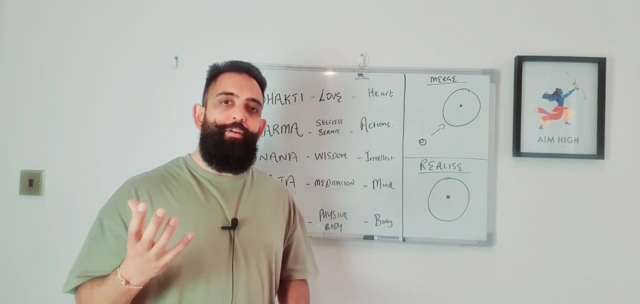 So, through Karma Yoga, you say that all the actions that I will be doing, I will be dedicating as an offering to the divine. essentially, I do not want the fruits of my own actions, And this is something that is very difficult to do, right? 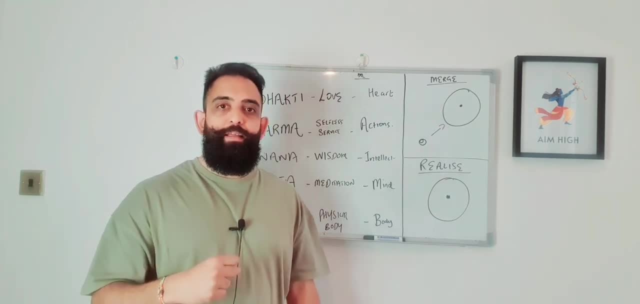 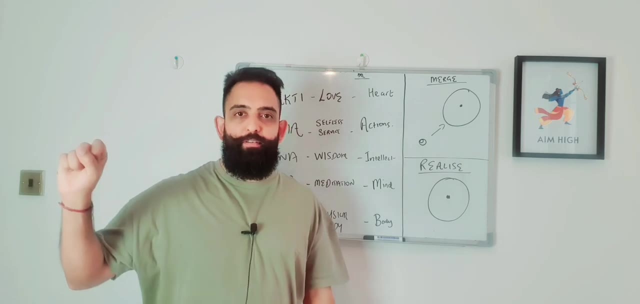 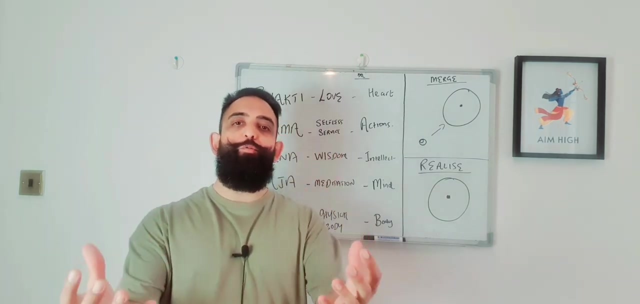 It's something that's very difficult to do, But ultimately, if we are able to do it, then we are able to get rid of the ego completely, And as soon as the ego goes, you realize that I am the universal consciousness. I am in you and you are in me. 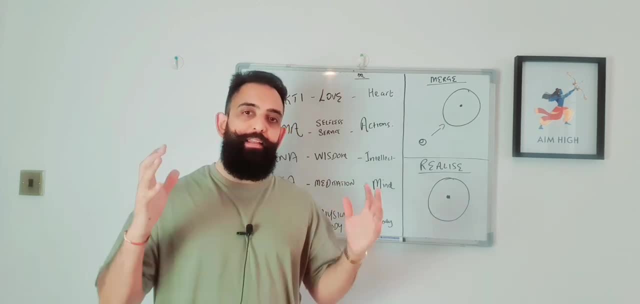 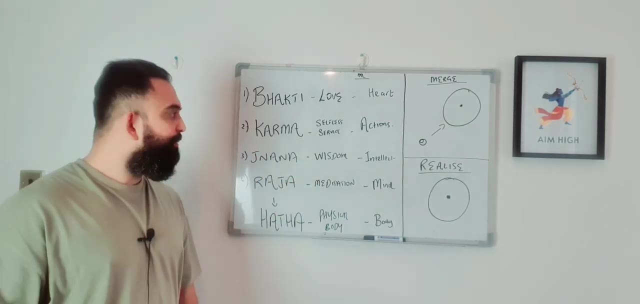 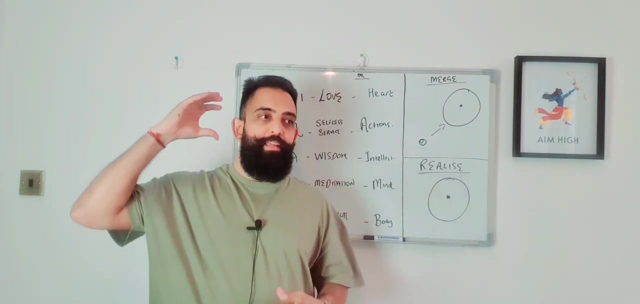 There is actually no separation. That separation was an illusion. So this is the path, This is the path of Karma Yoga. Then you have Jnana Yoga, which is the path of wisdom, the path of knowledge, essentially. So, Jnana Yoga, you are using your intellect, essentially, 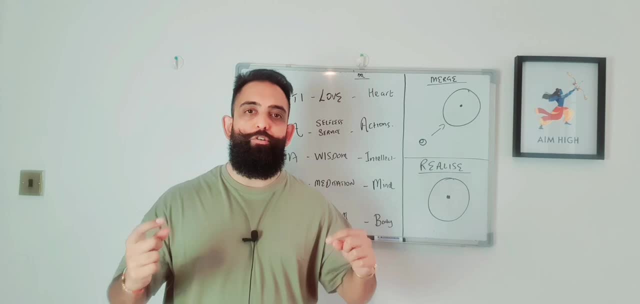 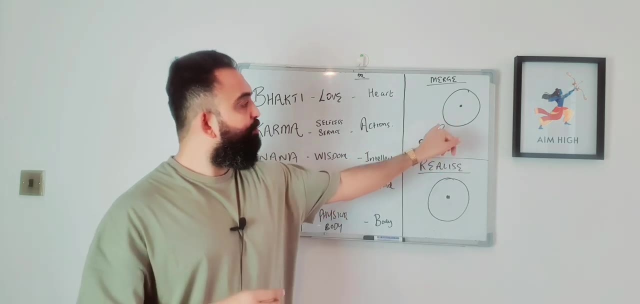 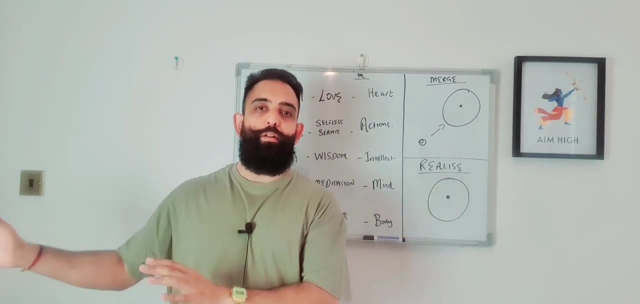 And you are trying to inquire into the nature of yourself. So if Bhakti is a path of merging the individual with the universal consciousness, then Jnana Yoga is actually the path of realization. So you are realizing that no, I am not separate, I am actually the all-pervading self. all is self realizing this. 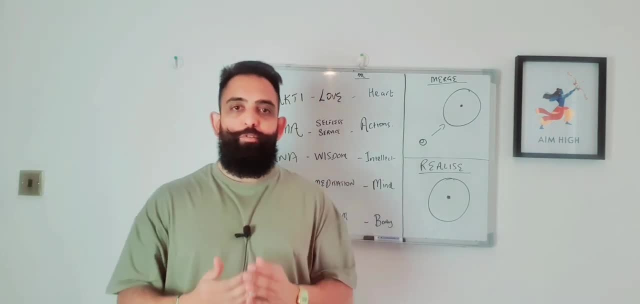 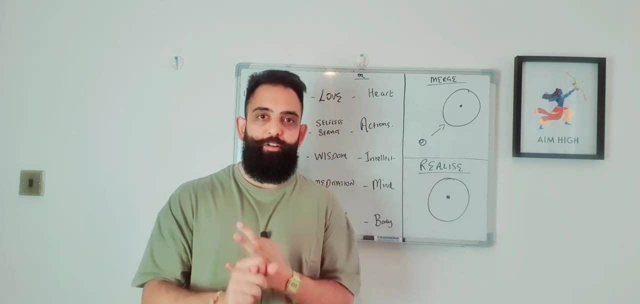 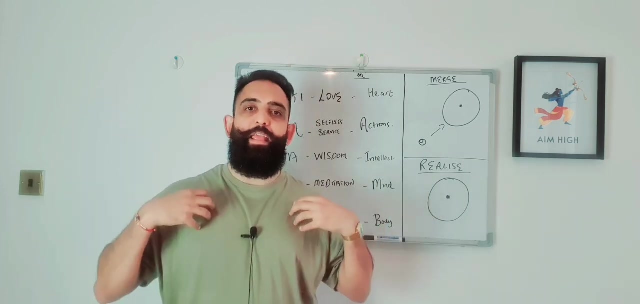 So the way that this is done is, first of all, through studying these scriptures: reading the Bhagavad Gita, reading Vedanta, reading the Upanishads, and really understanding what is the description given of this self. What does it mean? that it is all-pervading, that I am that. 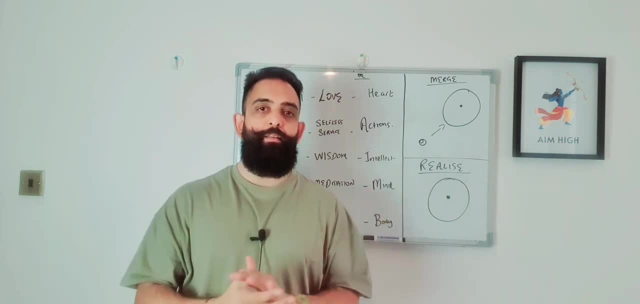 What does that mean, Soham? what does that mean? And once, alongside doing this studying, then you do practices of meditation where, for example, you can inquire into the nature of the self. You may have heard of the Who Am I? meditation. 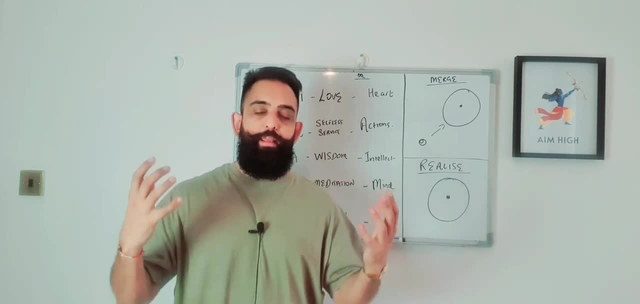 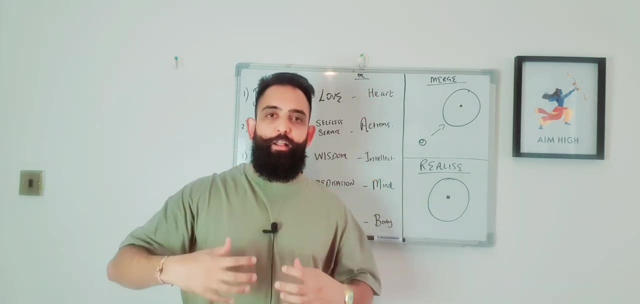 You keep on asking: Who am I, Who am I, Who am I? And you keep on negating the body. I am not the body, I am not the mind, I am not the intellect, I am not the prana, I am not the ego. 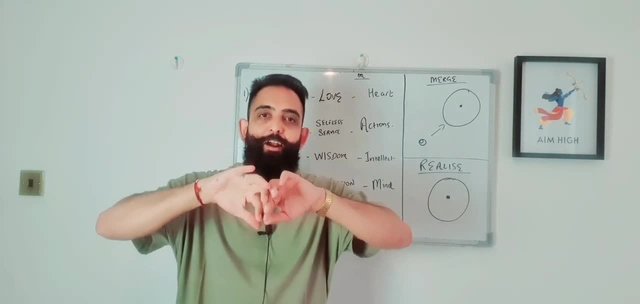 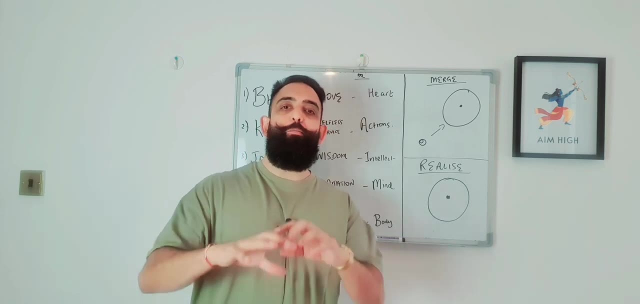 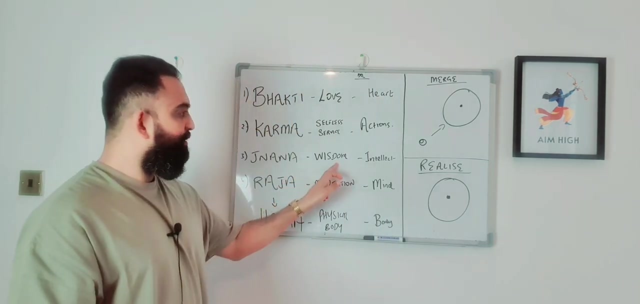 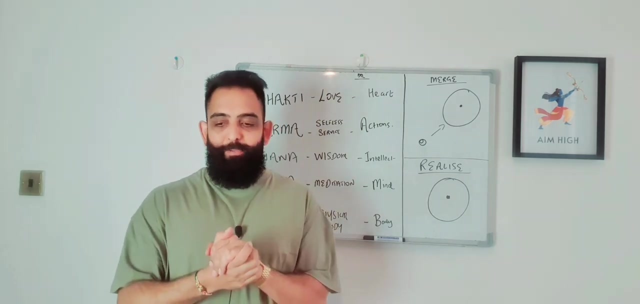 So what is remaining When you tear apart everything, when you go past all the layers? what will be remaining is the all-pervading, always shining self, And this is the path of Jnana Yoga, essentially. But remember that this is, although it is a very direct path, it is a path that can be quite dry. 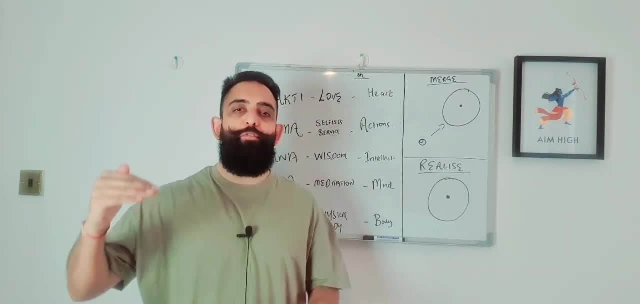 It is a path that requires an incredible amount of practice. It is a path that requires an incredible amount of practice. It is a path that requires an incredible amount of discipline- already An incredible amount of your ego. you know not being that big. 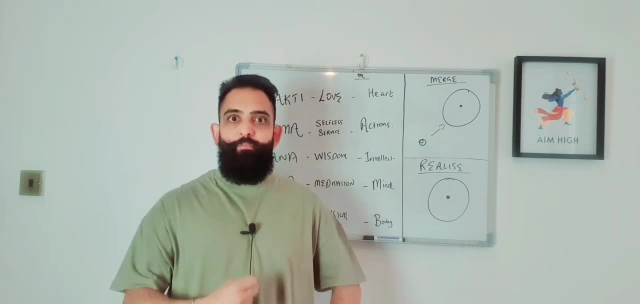 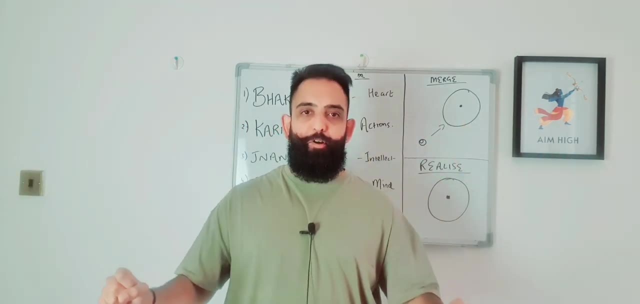 Because if your ego is prevalent, if your ego is big, and then you start to say that I am divinity, I am God, I am the pure consciousness, This will only make the ego bigger, taking you further away from self-realization. 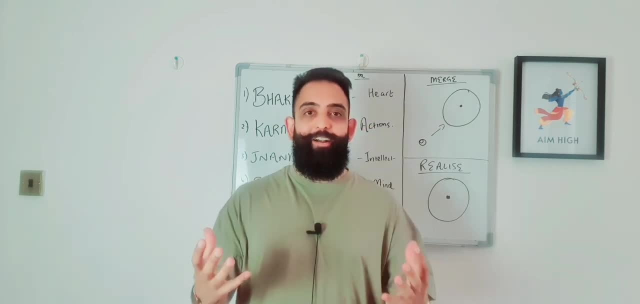 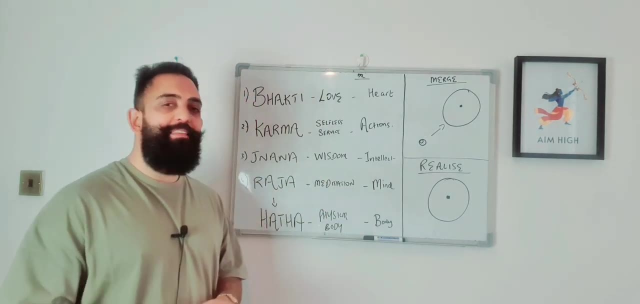 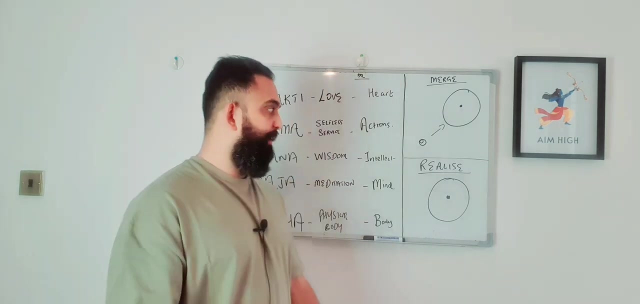 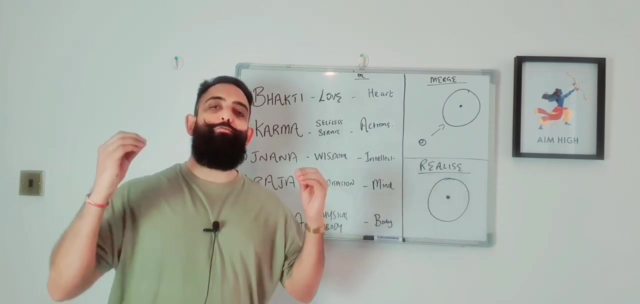 So it's really important to understand this. it's really important to know you know where we are before deciding to go all in 100% on that path. okay, and this is why you know working with a guru in who is practicing that helps, okay, all right. the next one is Raja Yoga. Raja Yoga is you know. Raja means king. it is the royal path. 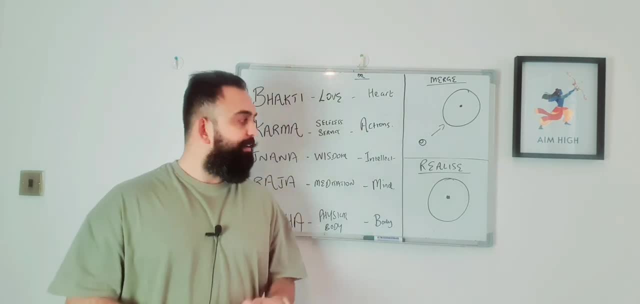 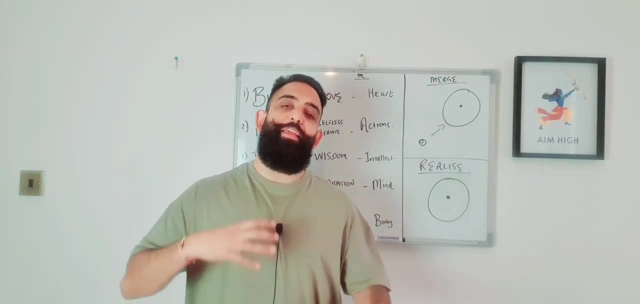 the path of meditation. essentially- and you know if you watch my videos- you've heard of the yoga sutras of Patanjali. The yoga sutras of Patanjali are the classical text for Raja Yoga, essentially. so here the premise is very simple. here the premise is that I cannot see or experience my 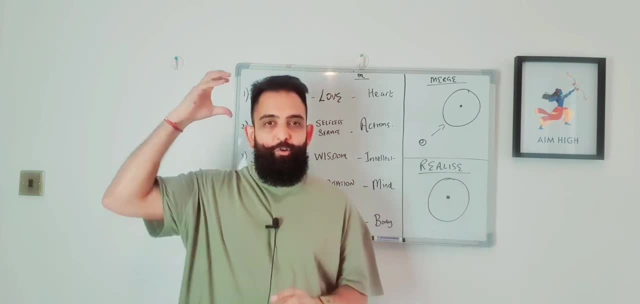 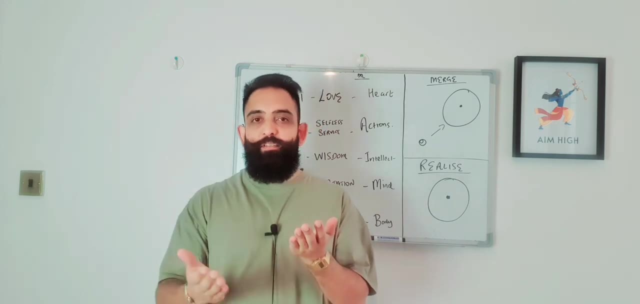 true nature because my mind has too much clutter. The example is given of the lake that has ripples on its side and I cannot see or experience my true nature because my mind has too much clutter. You cannot see what lies beneath, but the moment the lake becomes completely still. 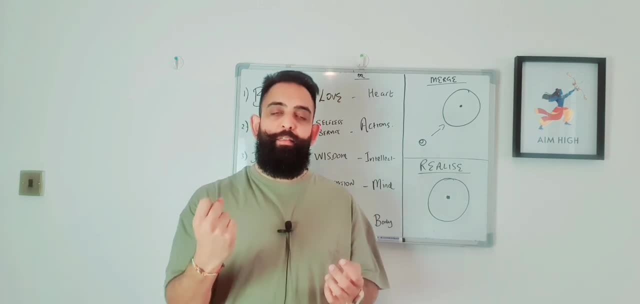 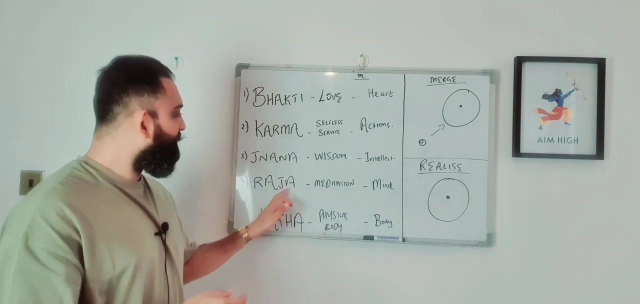 you can actually see what lies beneath. so just like that, when the mind is scattered, we cannot feel, experience our true nature. but the moment the mind becomes still, then what is within will naturally shine forth and realization of your true self will occur naturally. So here we are saying that because the mind is very scattered, through meditation, through 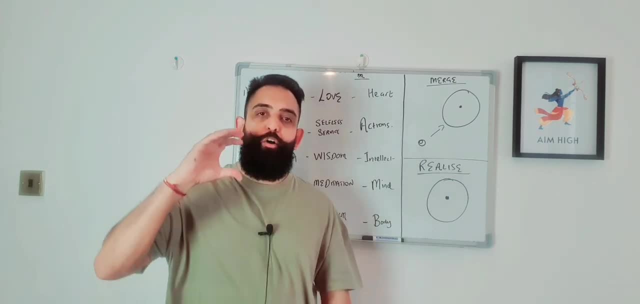 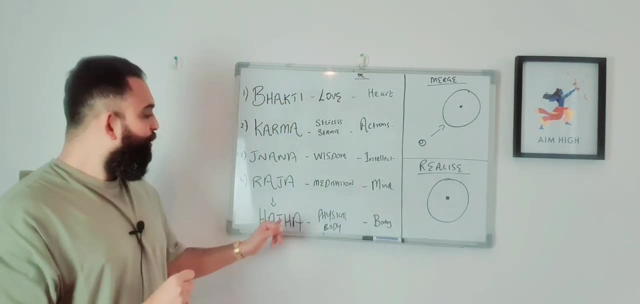 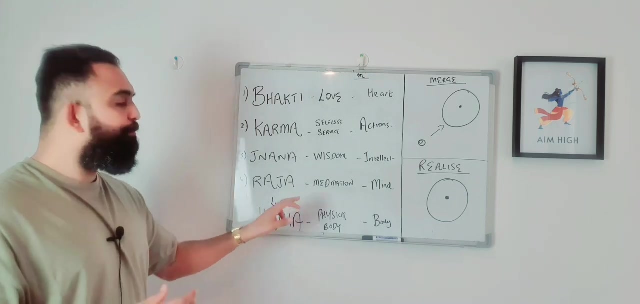 concentration. I am going to make the mind refined, concentrated, one-pointed and realize my true nature in this way. okay, and although not a part of these main four, Hatha Yoga, or Hatha Yoga, is actually a part of Raja Yoga. You can say that the purpose of this was to prepare you for the 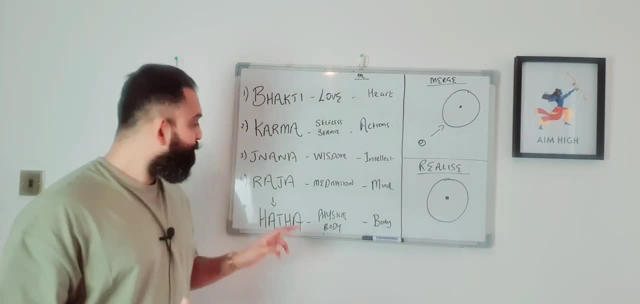 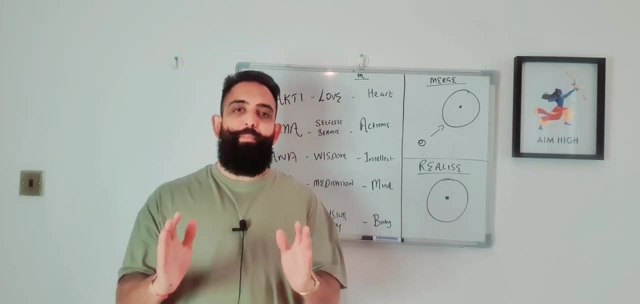 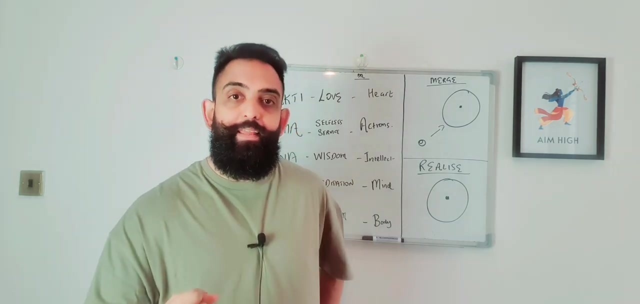 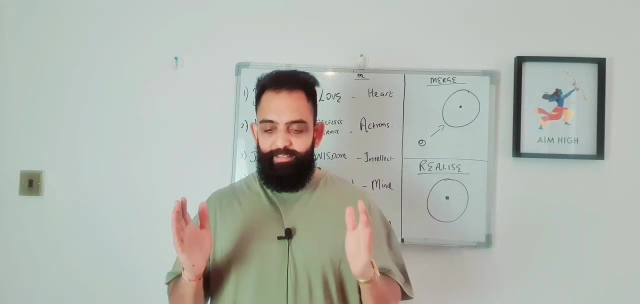 mind, the body for Raja Yoga. essentially because- think, think about it like this- to sit in meditation, to sit in meditation in the correct posture, completely still without moving, it requires some flexibility, it requires that your body is fit, in good condition to actually sit for the amount of time you need to sit for meditation, because we cannot do that. this 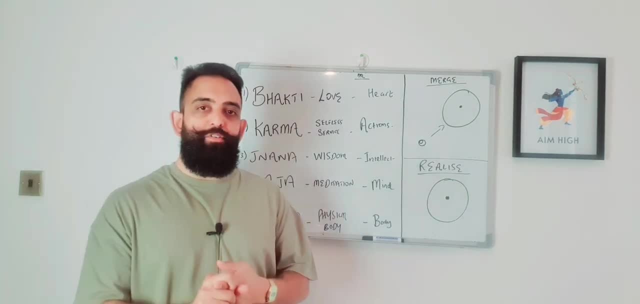 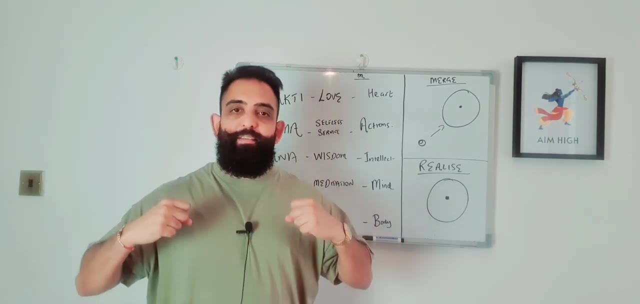 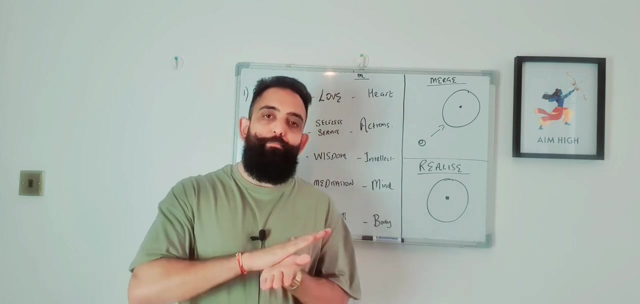 science has been developed, the yogic postures, the breathing exercises, it is all connected. so here, essentially, you are working at a very subtle level with the physical body, with the mind, with Prana, essentially, and what you are trying to do is you are trying to create a complete balance. 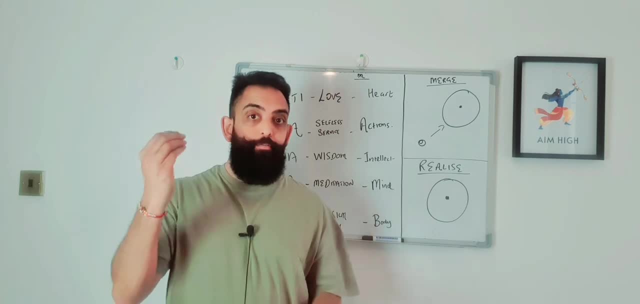 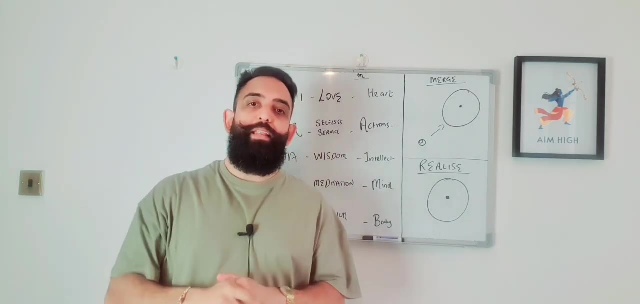 in the system and in fact there are many cases where just through Hatha Yoga, through raising your body, you can reach the top, most chakra. it means that realization has dawned. this is something that is possible, but of course it takes immense hard work and the lifestyles that we leave today. 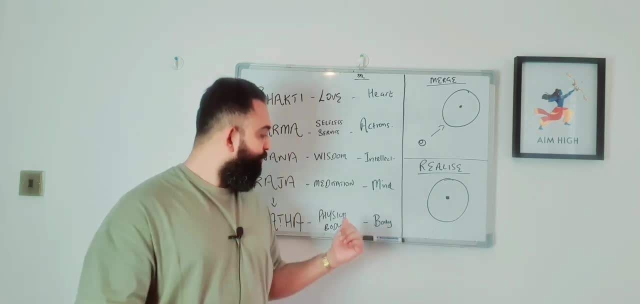 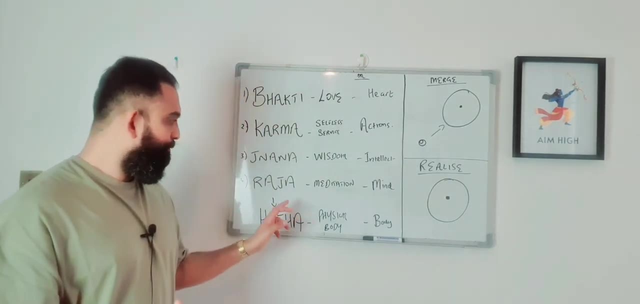 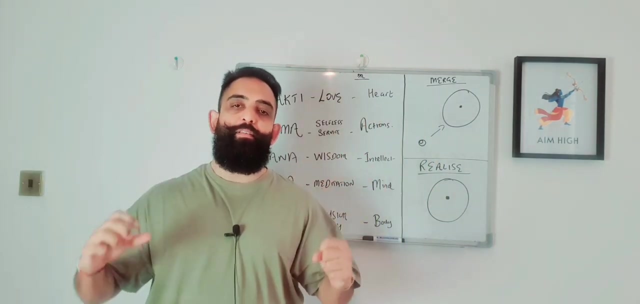 lead today are probably not conducive to having this as your sole path. so this is used as a stepping stone into Raja Yoga. so you first make the body fit, you make the breathing proper, and when this happens, you can then control your mind and you can then control your body and you can. 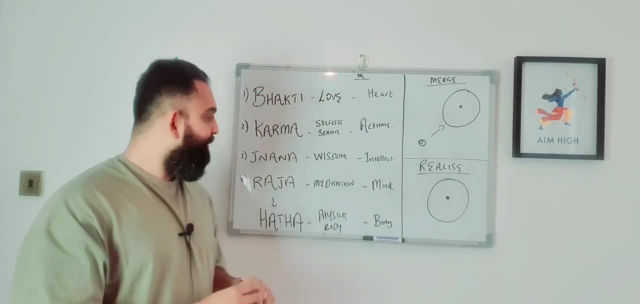 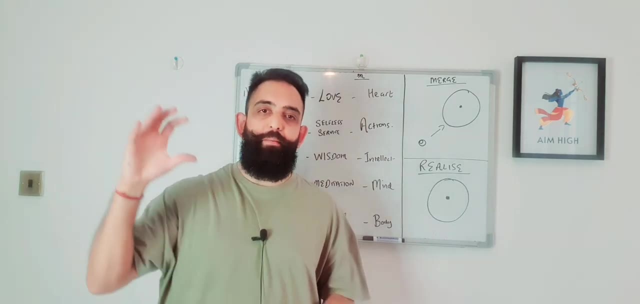 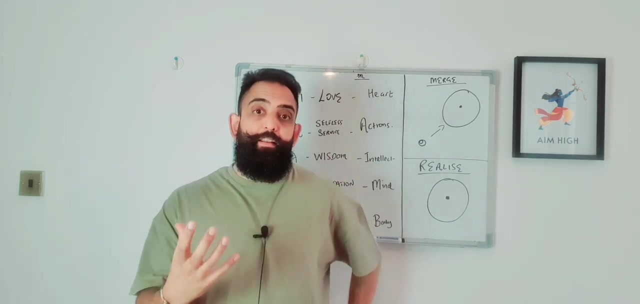 control the mind much easier. essentially so these two. you can look at them together. but ultimately, now that you have an understanding of the different types of yoga, one thing is really important to understand: that the greatest sages- take Swami Vivekananda, for example- have recommended: 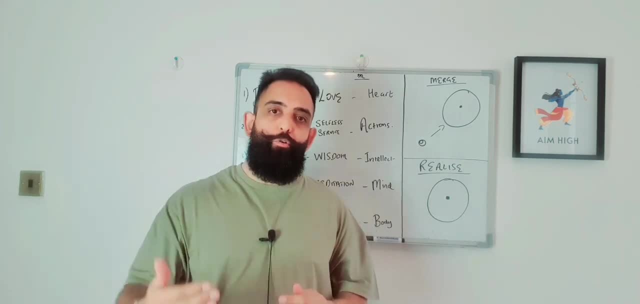 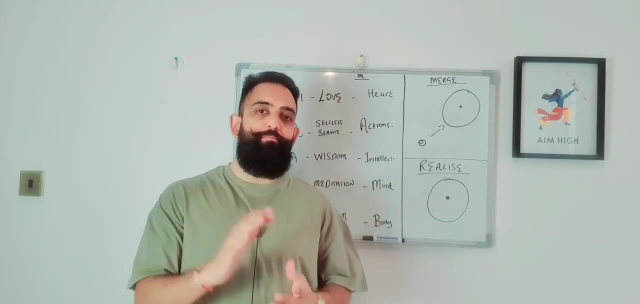 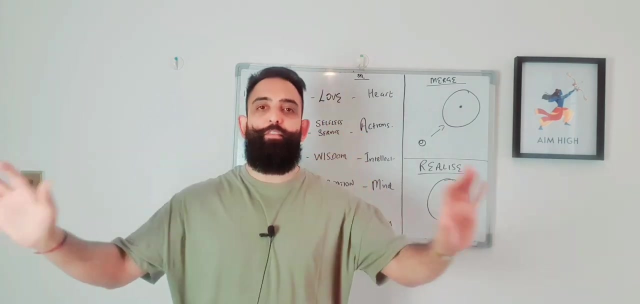 that we take an integrated approach of all four, not to just practice one alone. and let me give you an idea of why they say that. okay, so let's say that you say: bhakti is my part. I'm going to do just bhakti and nothing else. this has. I'm not saying this always happens, but there is a chance. 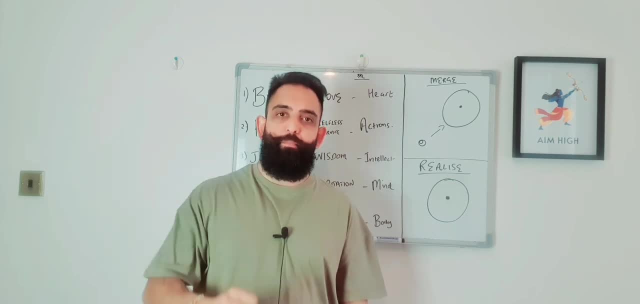 that it can lead to fanaticism of some kind, where you start to believe that the personal aspect of God that you are worshipping is the the only reality that you are worshipping, and that you are worshipping is the only reality that there is. and let's say that you were praying to Krishna and 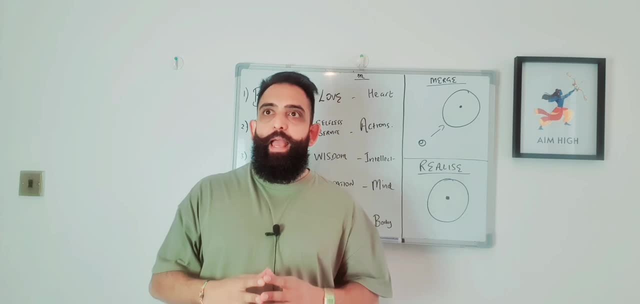 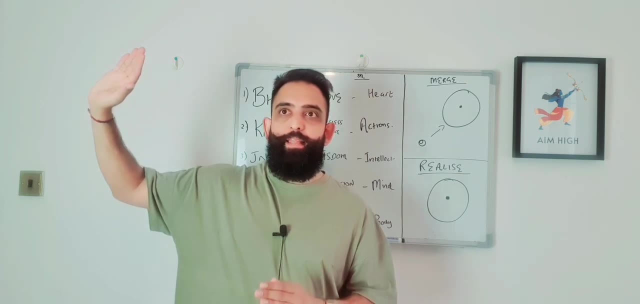 somebody else is praying to Allah, for example, right, different religion, and you may begin to think that no, this Allah is not. you know that is either not true, or there is a different entity, or you are not actually able to see that the Krishna that you are praying to is the same Allah, that the 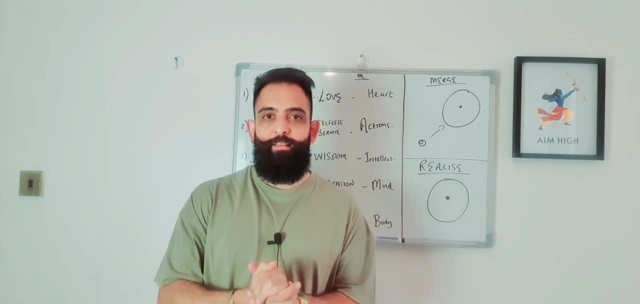 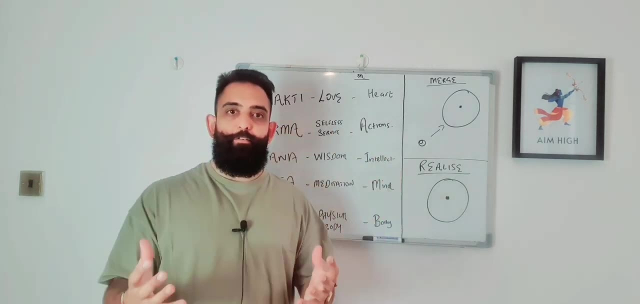 other person is praying to, because there is only one reality, right? so if you have knowledge of gana, if you have, if you have read that all itself, if you have understood that there is only one reality, you can give it any name that you want you can have. 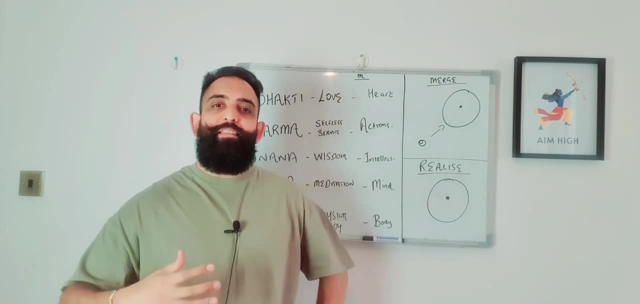 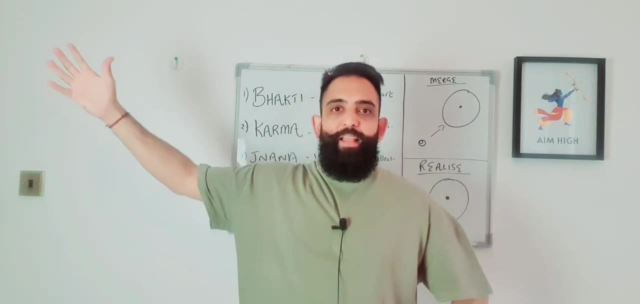 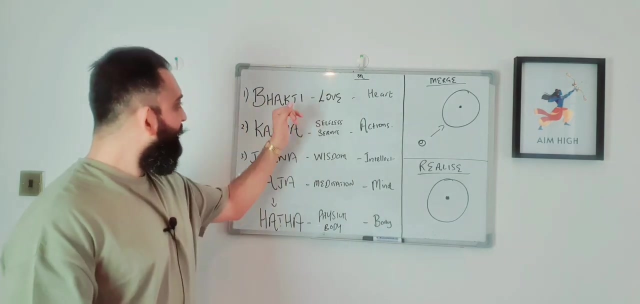 a personal God of your choice. but that is just a support essentially for you on the path. it doesn't mean that if somebody else is doing something else, that it's that that you know has less weight or carries less weight. do you understand? so, having an having an integrated approach where you know you can, you can focus all. 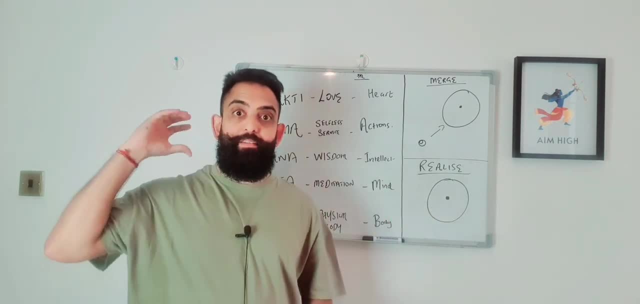 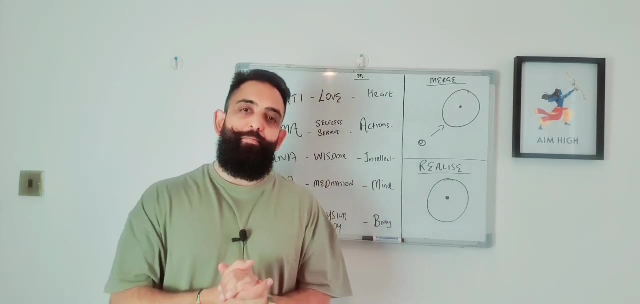 of your love on one deity, no problem. but at the same time, knowing that if somebody is praying to a different version of god or a different aspect of god, it is ultimately the same. it is the same supreme that is being prayed to. it is not different. so, bhakti, when you are doing bhakti, 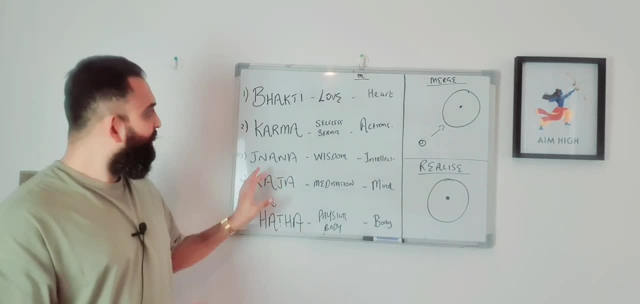 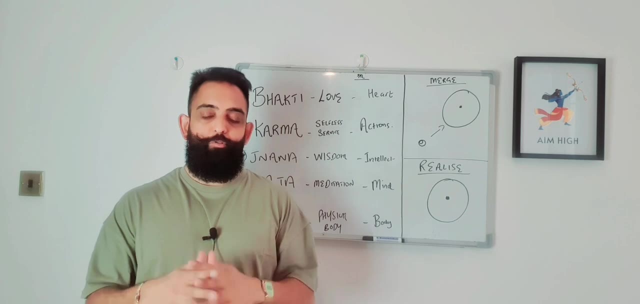 ghyana is also important right, and there are many different examples of all of these. ultimately, you know, they all need to be integrated. they all need to be integrated for us to have the best chance, essentially right. i'll give you another example: karma yog, right, karma yog, the. 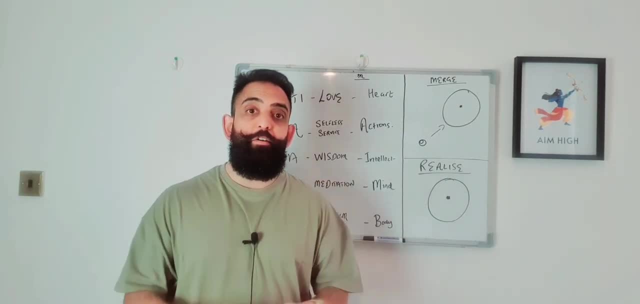 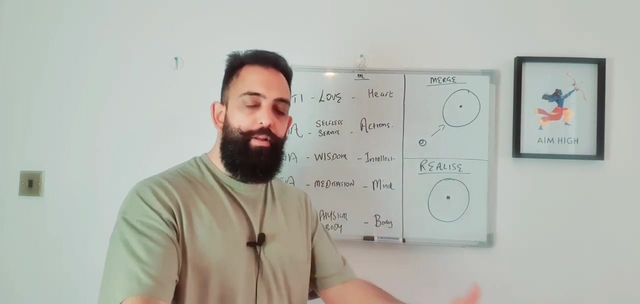 path of selfless service. so you see so many people that you know begin with very, very good intentions, a charitable organization to help others out there, and what begins to happen is that organization is an organization that is a responsibility to help others out there. organization grows and that person goes from serving people on, you know, the, the streets or 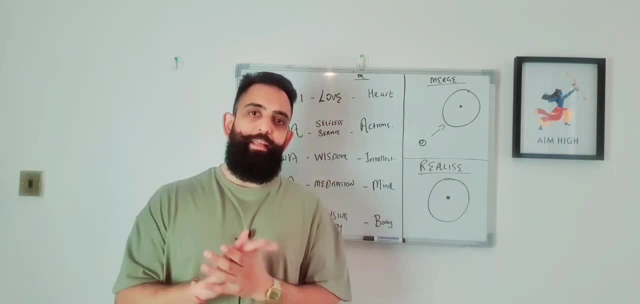 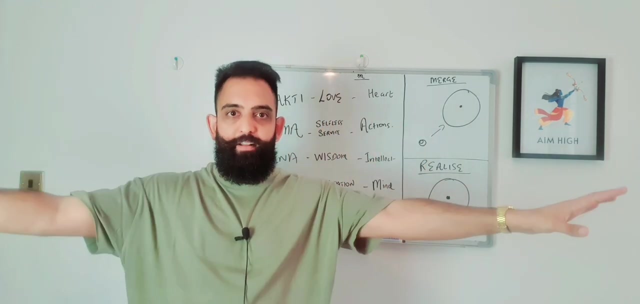 actually physically serving people to now arranging other things. now they're trying to arrange meetings with this NGO and that NGO and having international meetings and all of a sudden, you know this person has become a charity superstar and the mind has become completely extroverted. so what was actually supposed to make you, you know, diminish the ego, is actually now. 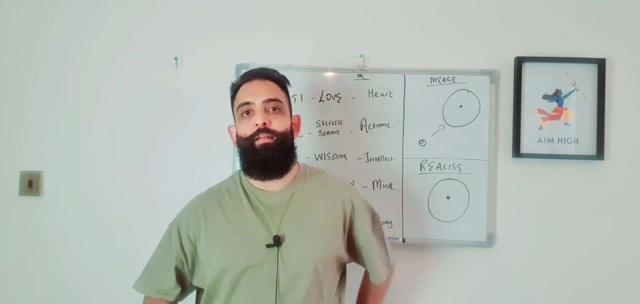 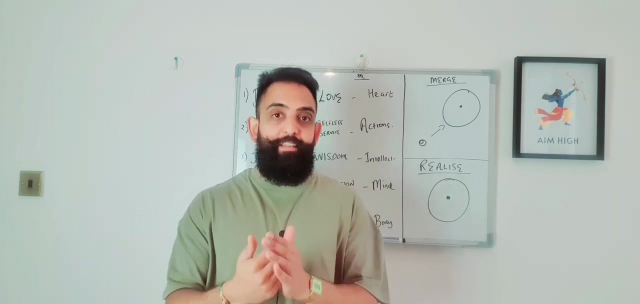 increasing the ego because your organization has become so big. so it is always important to realize that, no matter what path we take, we are taking it for a specific goal and to reach that goal, the ego needs to be completely demolished. essentially, it needs to be completely demolished.